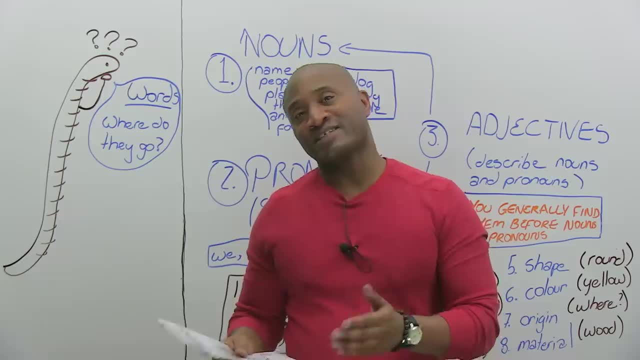 word order. Where do you put the words in a sentence? In some languages they have a different word order. Some languages, it doesn't really matter, But what my job today is is to show you where the words go, and what do they basically mean. Okay, In the parts of 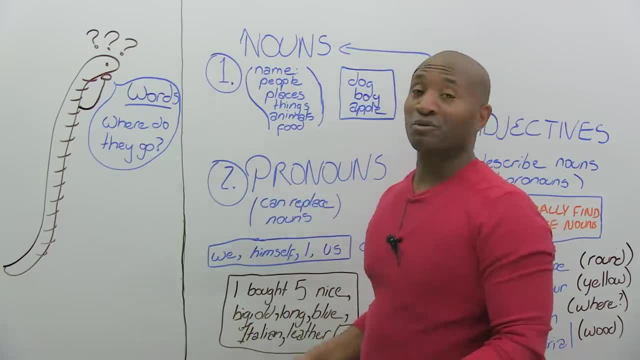 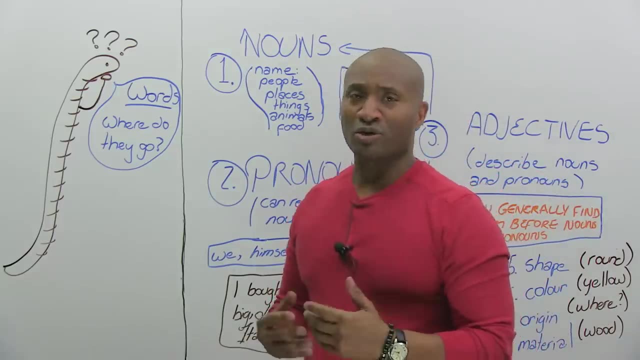 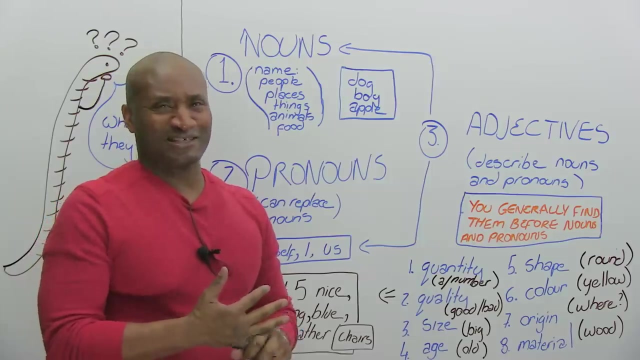 speech. As E said words, Where do they go Now, if you're new to English, or even if you're an intermediate student, sometimes this causes you problems. Right, You've heard the terms preposition, determiner, syntax and you're like, oh, it's so complicated. 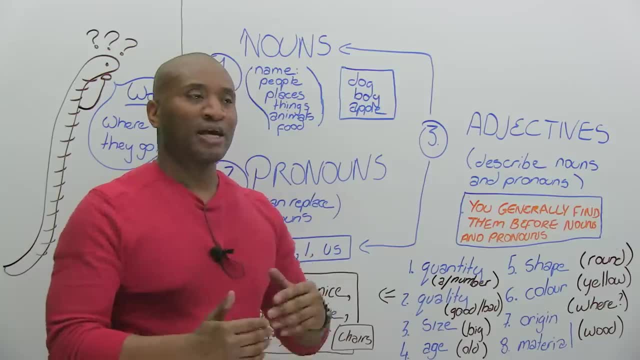 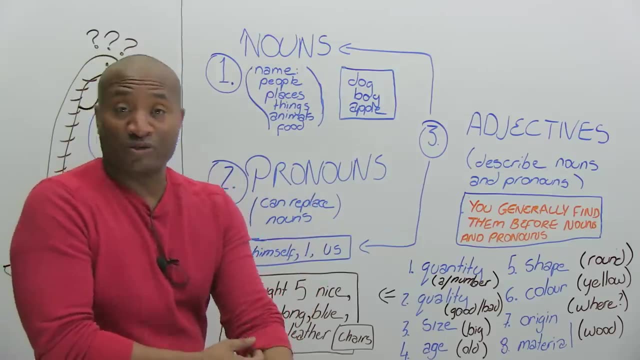 Today's lesson will be simple. You can go over this again and again. It will help you understand and use English better. So I'm going to start off with the most basic part of parts of speech And I want to start with the things part. Things, Not actions, but 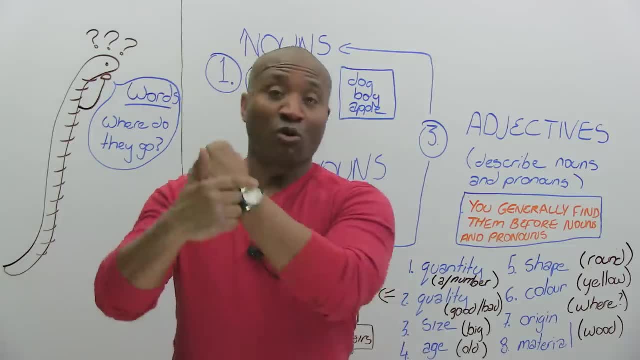 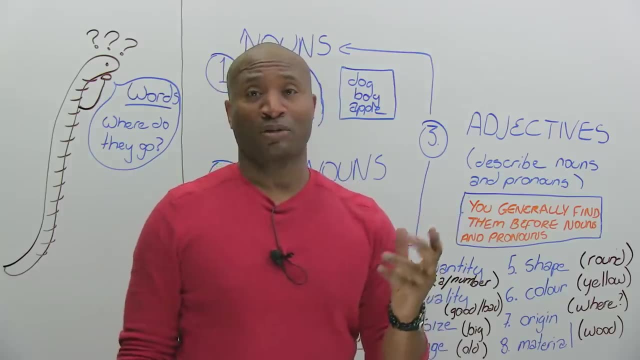 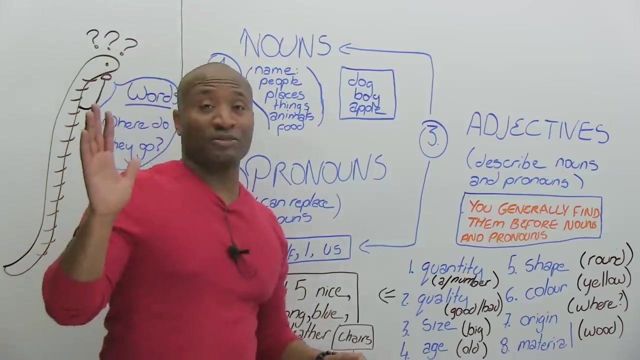 things. I am a person, My watch is a thing. Okay, An animal, a cat or a dog or an apple. These are things. We call these things nouns, Because nouns name people. Hi, I'm James. Places, Toronto, Ontario. Things my watch. 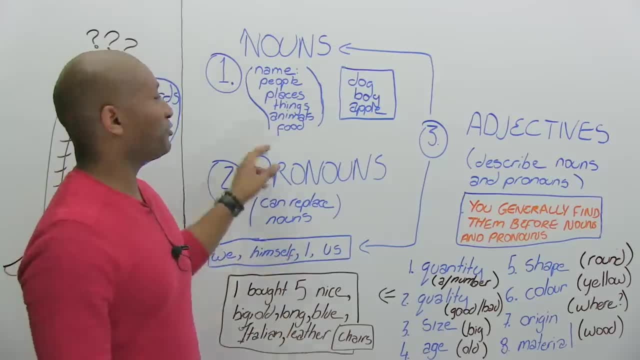 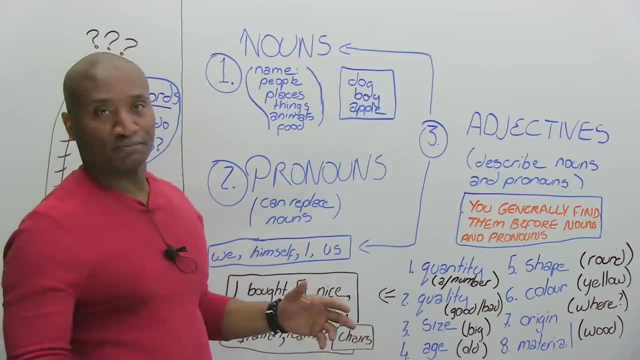 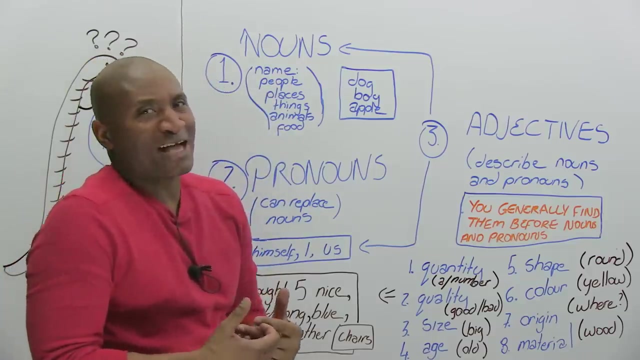 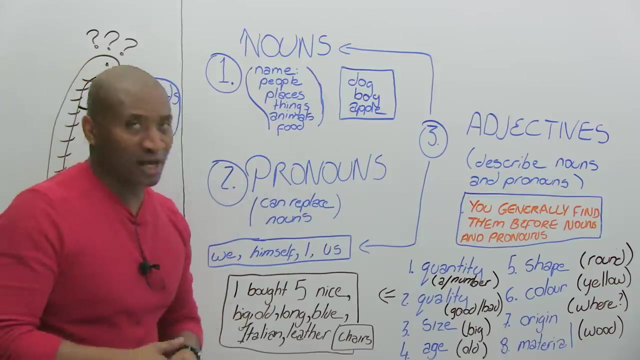 animals- a cat- and food- an apple. Okay, These are nouns. Example: boy, dog, apple. Nouns name these things, But sometimes you don't want to keep using the same noun again and again. James ate the apple and James walked his dog as James talked to his friend Oliver. 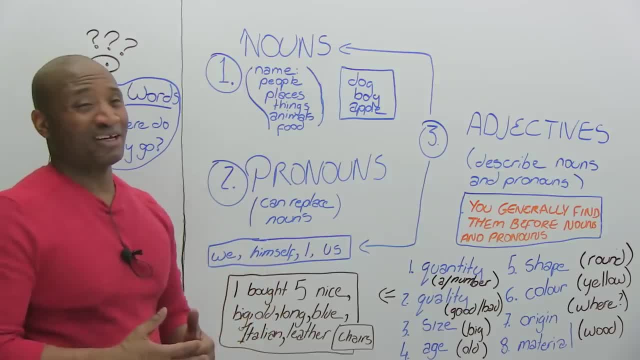 And then, James, it gets what we call repetitive and boring and also makes the sentences go really slow. And sometimes we want to use the noun in a different way. So in this case we introduce what's called pronouns. Pronouns can replace nouns in a sentence, So now you could say something like this: 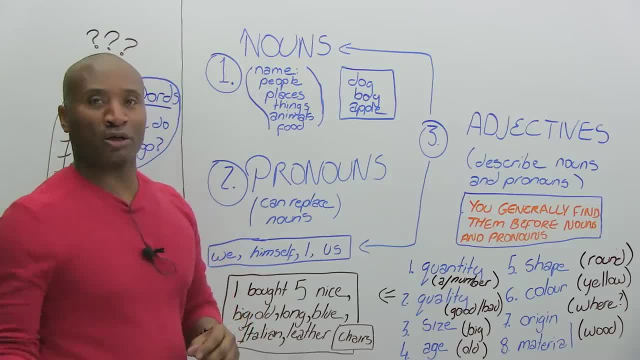 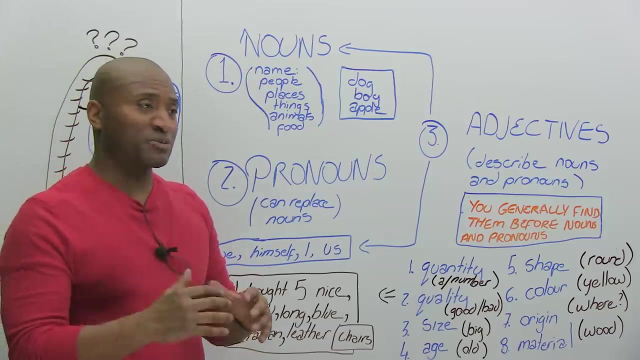 James ate the apple and he walked his dog. Instead of James ate the apple and James walked his dog, we can use a pronoun to replace it and make it simpler. We still know we're talking about James Now. we talked about word order or syntax. Let me explain this. 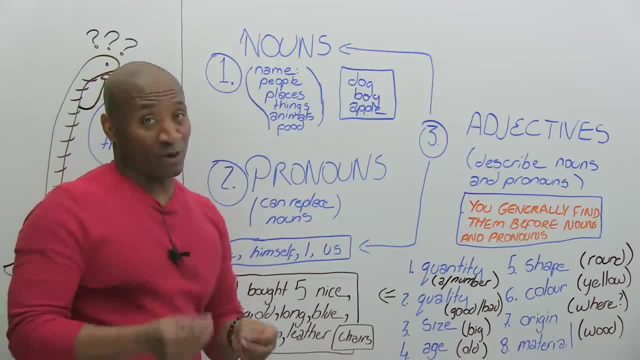 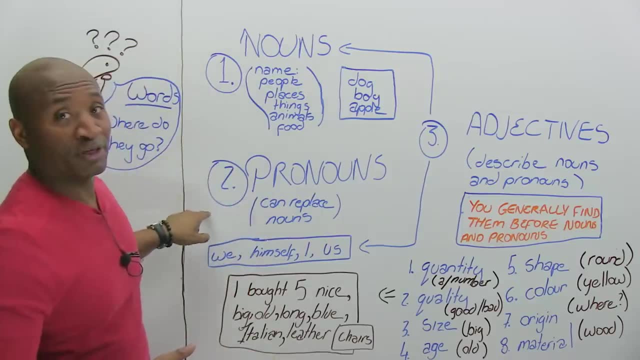 In order to use a pronoun, first you must use the noun. Okay, You introduce the noun and then you can replace it with a pronoun. That's why you see number one and number two. You cannot just start with a pronoun. If I started a sentence at the beginning, he went. 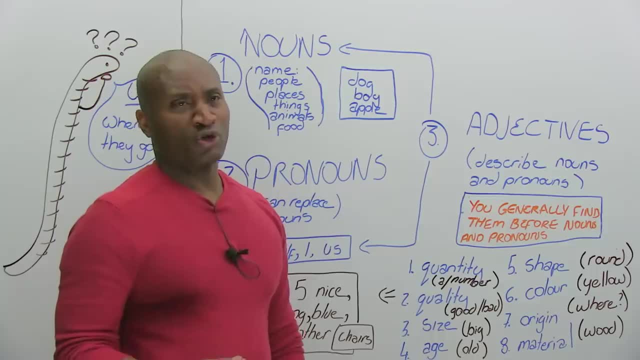 to the store, the very first thing you'll say to me is: who's he? I go, oh, James went to the store and he bought the apples there. And you go, oh, now I know who he is. So 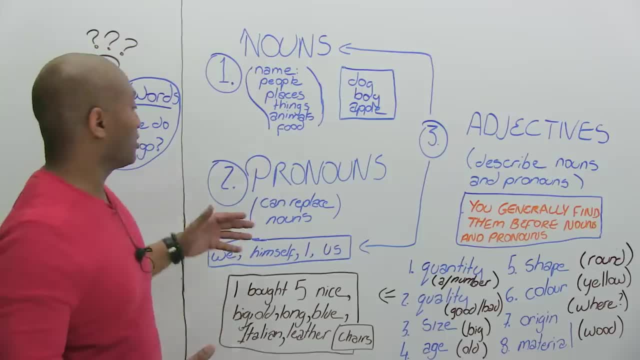 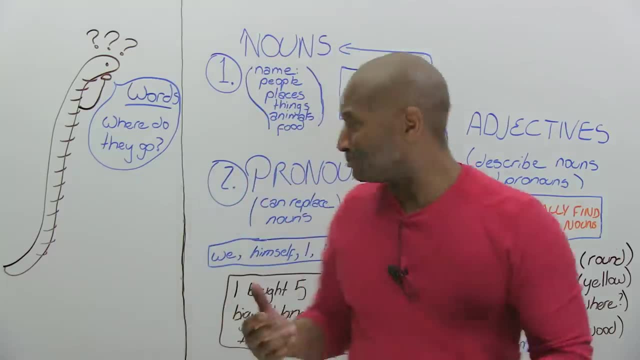 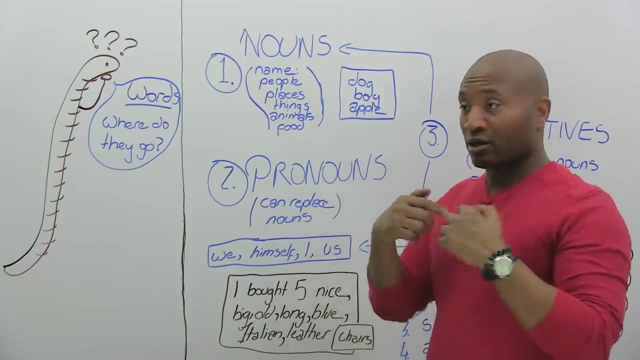 pronouns come number two, because you have to actually introduce first with a noun, then you can replace it with a pronoun. Now we have several types of pronouns. I'm just going to go over and show you a couple of them so you get the idea. Pronouns include I, we. 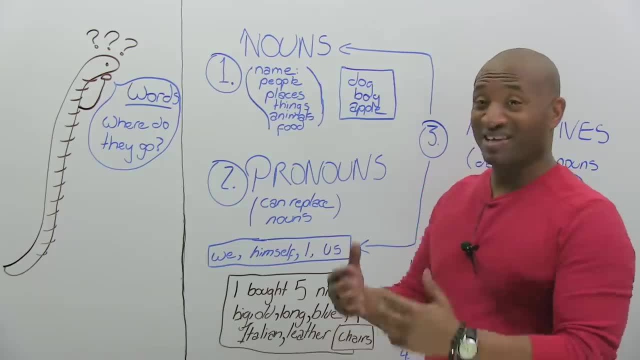 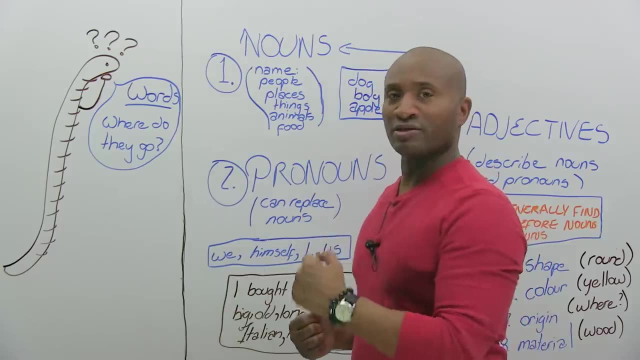 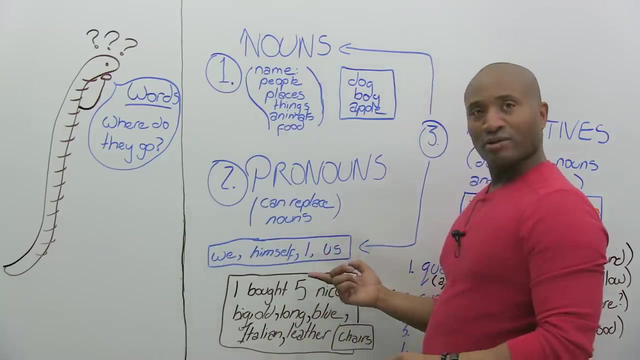 which are subject pronouns. Object pronouns when we're talking about something that's not us, but something on the other side that receives action as a subject pronoun. I do things, I run Right, We eat dinner, We're talking to them. Now, when we say them: you go, what? 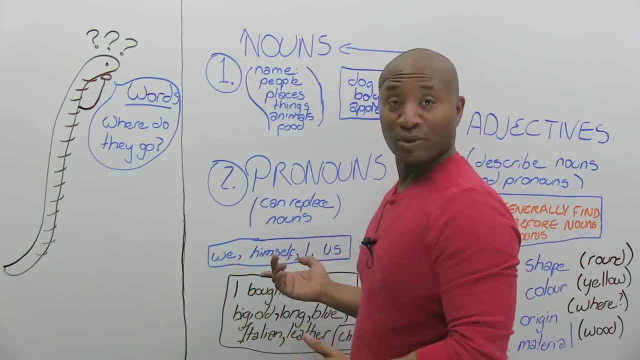 Well, they are receiving it and we'll call those object pronouns. Okay. So the most basic ones are subject and object pronouns. One is doing something, one is receiving. There are reflexive pronouns, like himself, where somebody is talking about themselves. 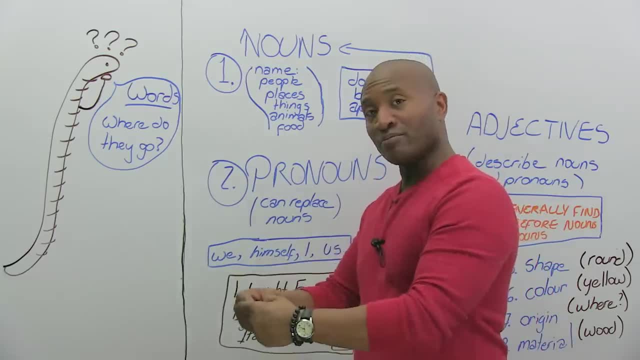 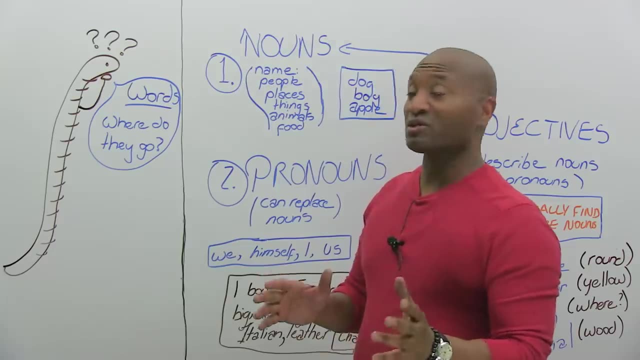 He built the house himself, So he's talking about him as an object, but reflecting it back to himself. We call it reflexive pronouns. Okay, There are others, but I'm not going to get into them right now because I want. 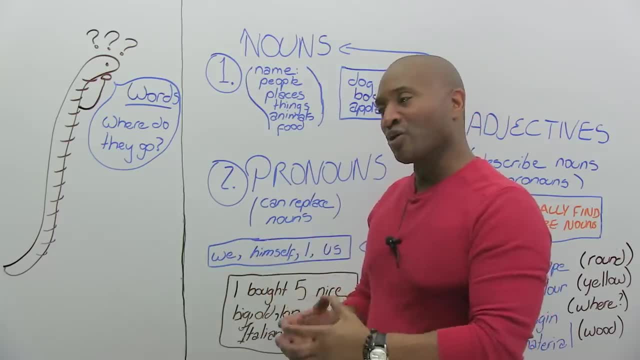 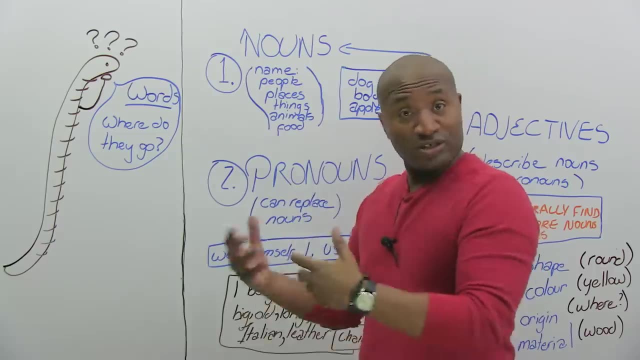 to keep this simple, just so you know what the parts of speech are, and you can always come to engVid to come and see other lessons in which we go deeply into reflexive pronouns, object and subject pronouns. Okay, Cool, So we've talked about how pronouns can replace 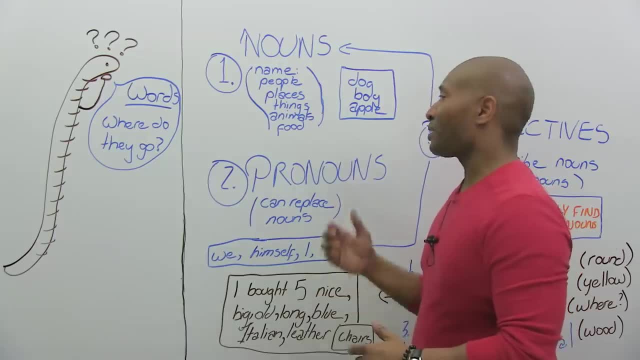 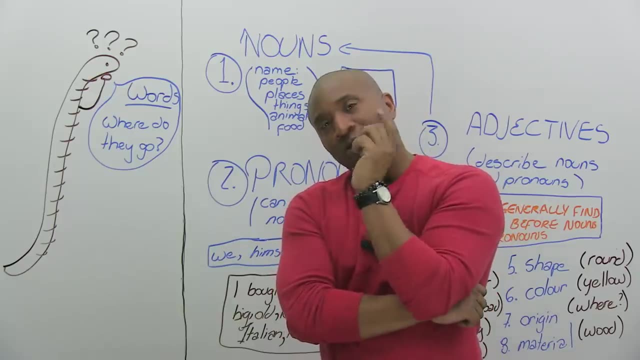 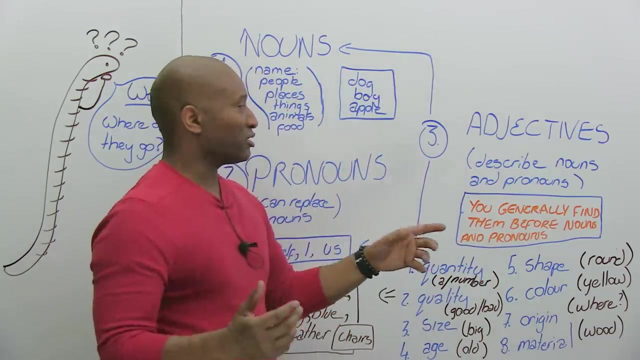 nouns, and we're good with that. Yeah, So let's go to stage number three, because once you've replaced them, how do you know the difference between them? Apple, apple, I don't know. That's when we have adjectives- Adjectives- The word itself can be broken into two parts. 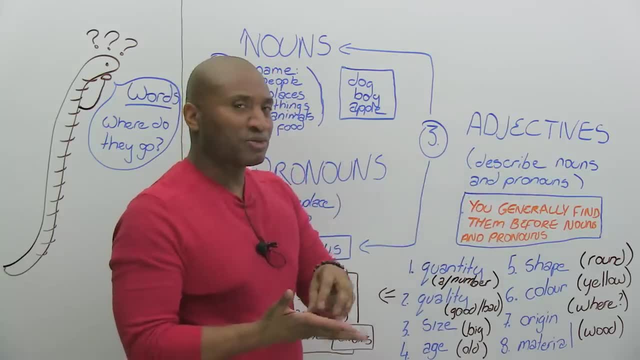 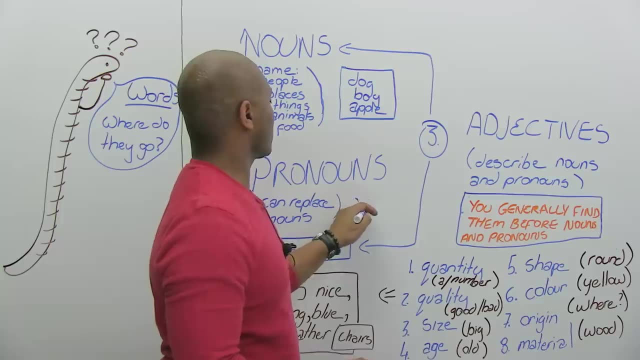 Object and ad. Do you remember when I said subject and object and I gave you the example? I said, for instance, I is a subject pronoun Right. Subject- yeah, I'm good at this, I do this really well- And I said: them is an object pronoun Right. 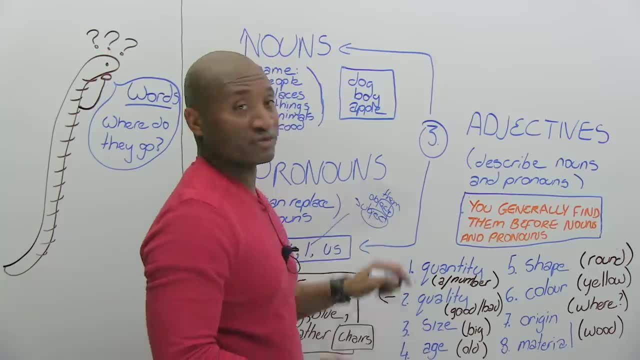 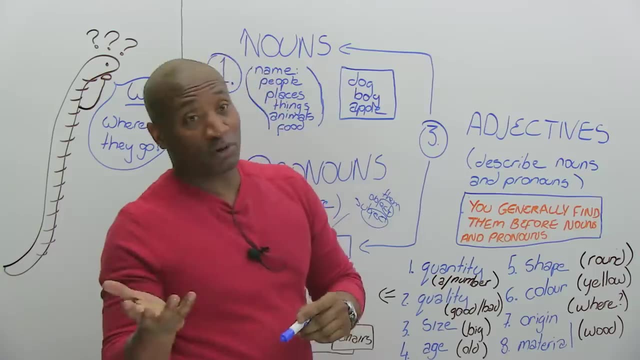 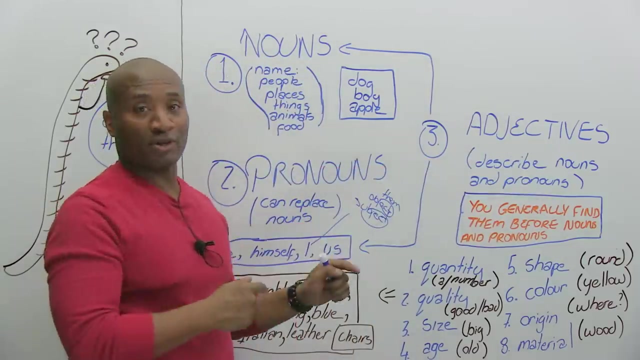 You'll notice object is in both parts. When you look at an adjective, add means to put on. You add like two plus two is four, Four plus four is eight, So an adjective you add to a pronoun or a noun to describe them. So if you look here object adjectives describe 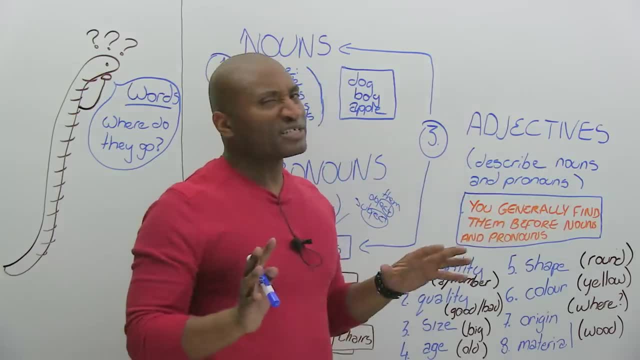 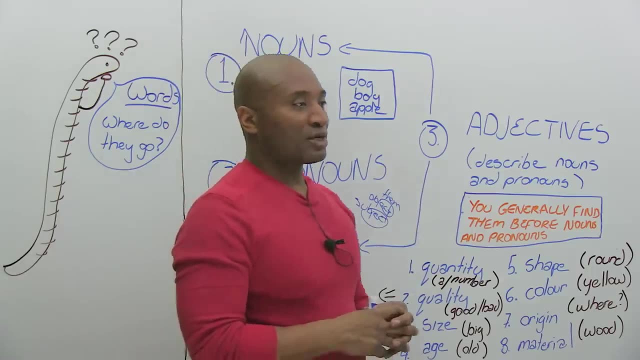 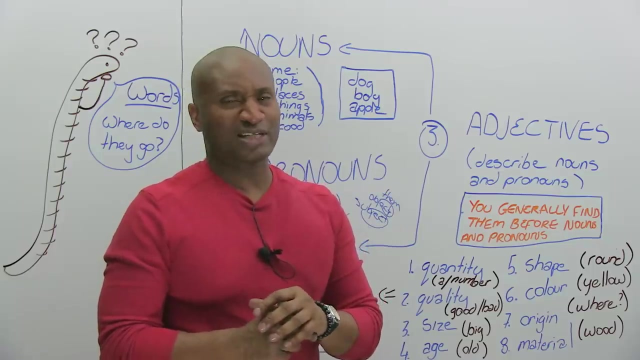 nouns and pronouns. Now, remember, we talked about syntax. Well, syntax, remember the word order. Where would you find an adjective? Well, in some places it's reversed. If you speak Spanish, for instance, you would say gato negro, which in translation for English is: 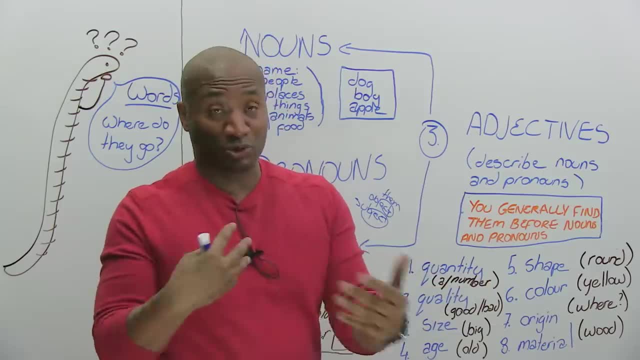 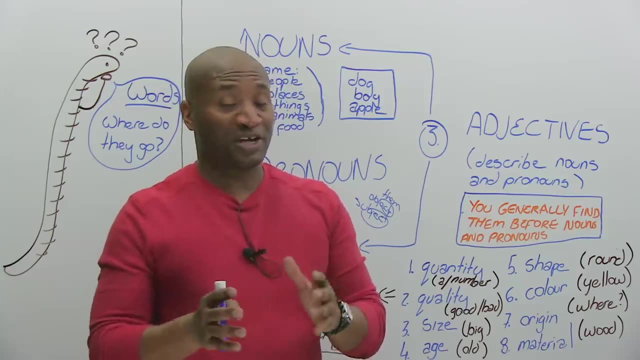 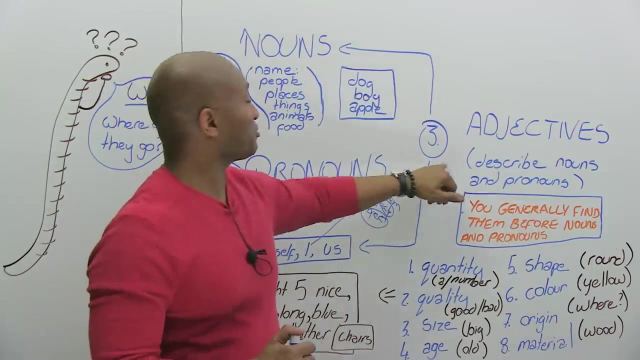 cat's black And for me who speak English, or a person who speaks English, that doesn't make sense to me because we say black cat. So word order can vary depending on the language you speak. We usually put pronouns before Sorry, adjectives before our pronouns, and. 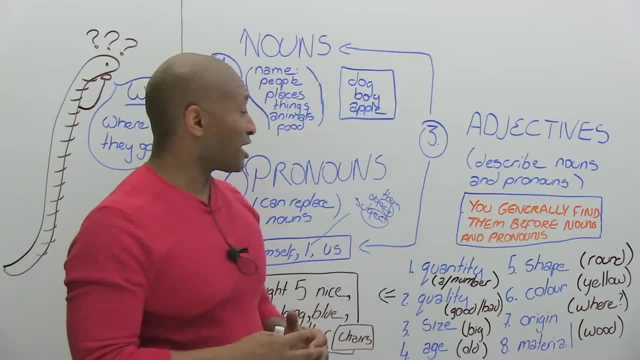 our nouns so we can describe them, And in two seconds I'm going to give you some ways in which we describe things and we have a word order for that. Okay, And I'll have to explain something on that. So where will you find an adjective Before you find your? 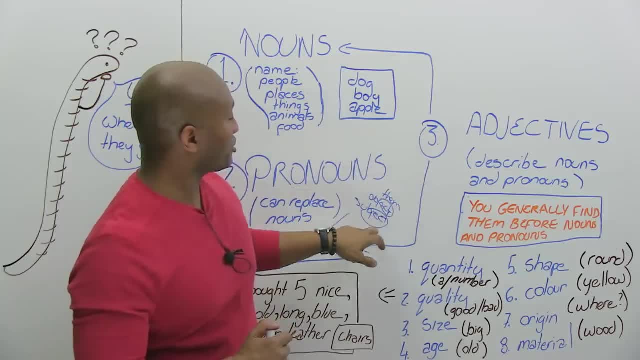 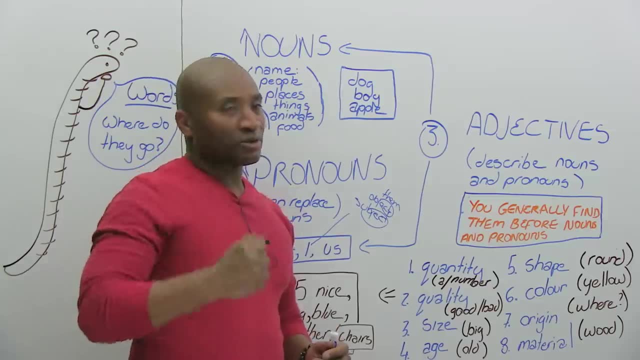 nouns or pronouns. They will help you describe your subjects or objects. Okay, The things that are doing something. Now we have eight types of adjectives, All right, And we have a special order we put it in. We put it in the subject: the subject, the object, All right. 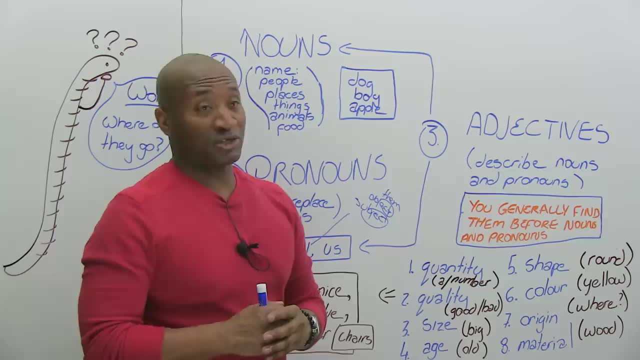 I'm going to give you a little bit of a list. first, I'm going to give you a list of the put it in Now. depending on your language, this order may exist, you may have a different order or you may have no order, which means you can put any of these things in any order you. 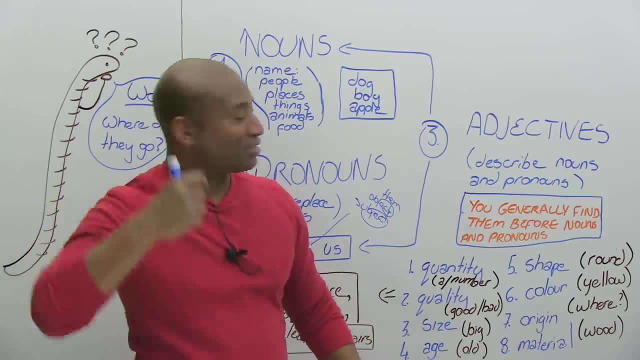 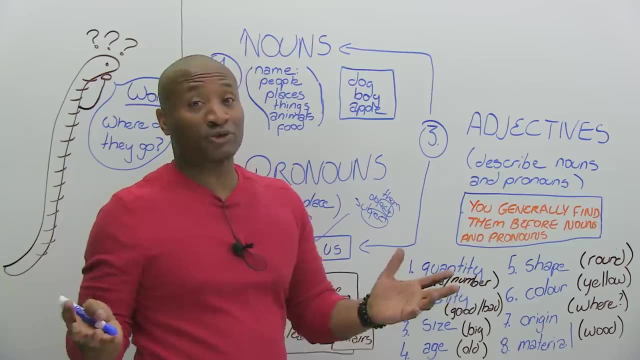 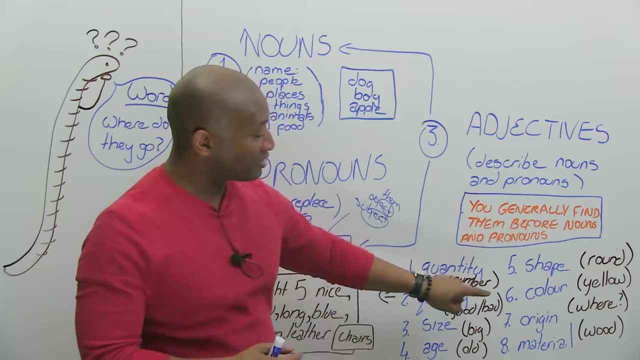 like You can put. Well, maybe with the exception of numbers, but the colour can come first, where it comes from, it can come first. the quality can come first. it depends on your culture, your language, your country, English. however, the order I put it in one, two, three, four, five, six, seven, eight. 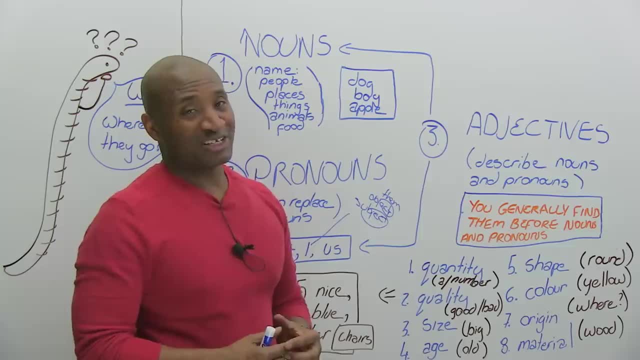 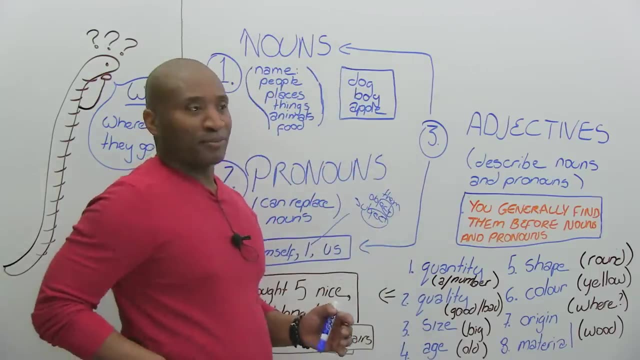 that's the order we want it in, Okay. If you change it, it actually gets really confusing. So what are these eight? Why don't we take a look? Quantity, it's a number. Now, I put a number not because I said a number, but a refers to. 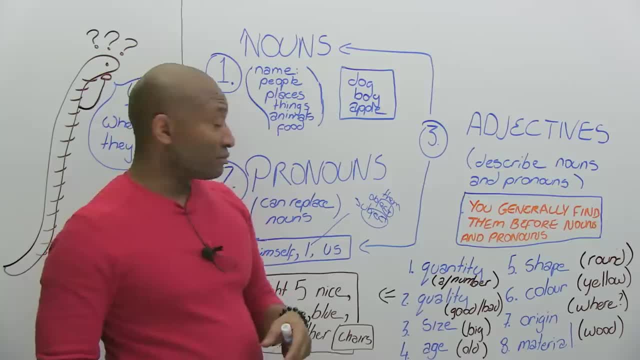 Or a refers to articles. The chair: a chair, Okay, In this case a means one. so that's why I put a number. Funny guy, I know, Number can be any other number: Five, ten, one thousand. 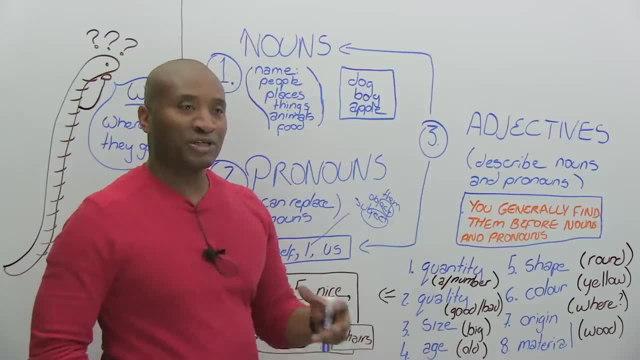 One million A billion. This usually comes first to indicate how many things we're talking about. Okay, So you need a number: Five chairs. Okay, I'm talking about five, so I have to look for five chairs, not chair yellow five. 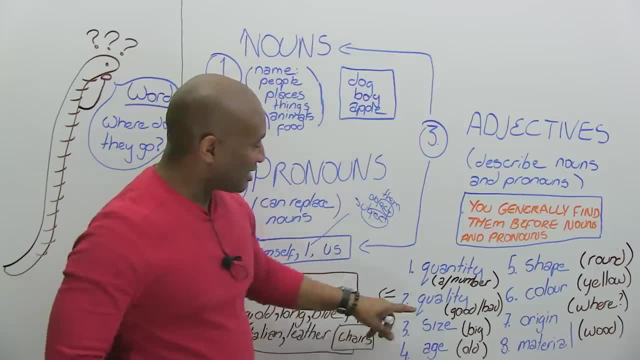 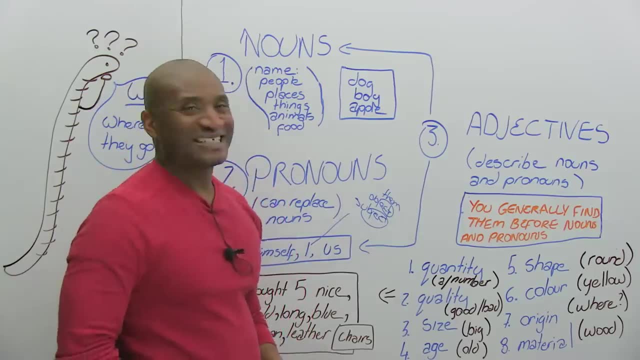 I'm like: oh, is that the name Yellow five? I'm confused. The next thing we talk about quality. Is it good, Is it bad, Is it exceptional Right Or is it insignificant? That's a big word for meaning, not important. 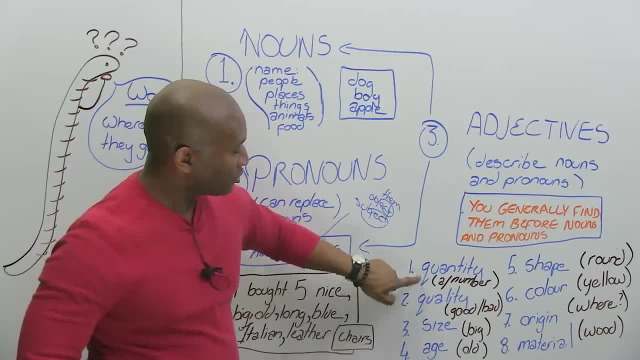 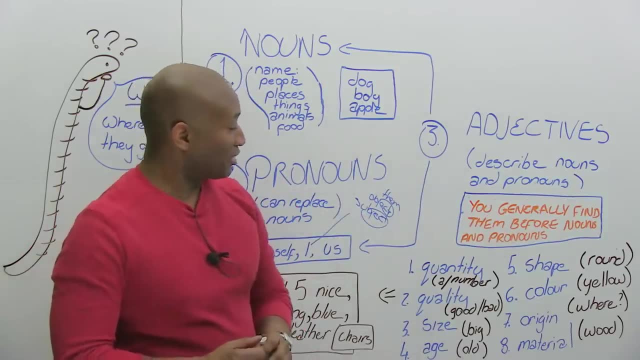 Okay, So we go from quality to sorry, quantity to quality. Then we talk about the size of it. Right, There were five big black cats. so five big. Is it big? Is it small? Age: How old is it? 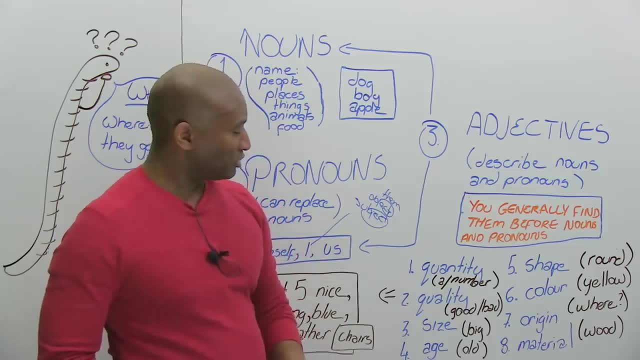 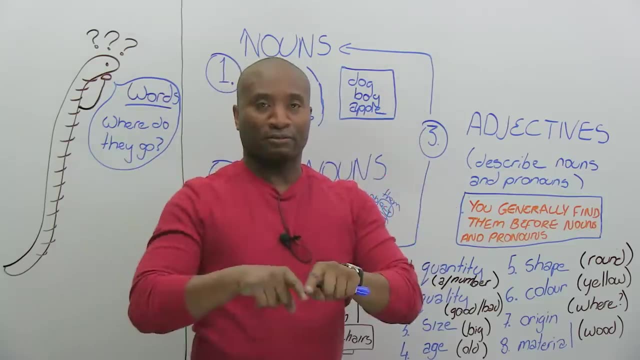 Is it new, Is it old, Is it young? Right Shape, Is it round? Is it a square Or a triangle? What's that? What's the shape of it? Oblong, Yeah, that's Don't. 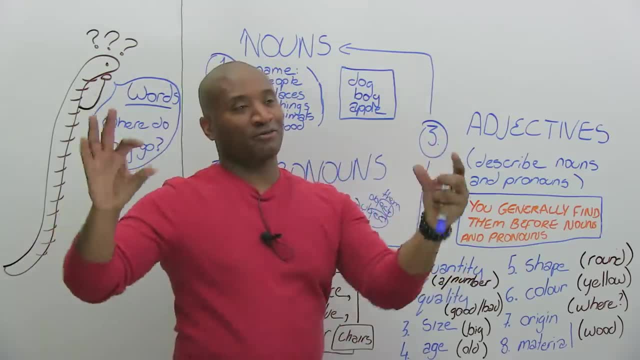 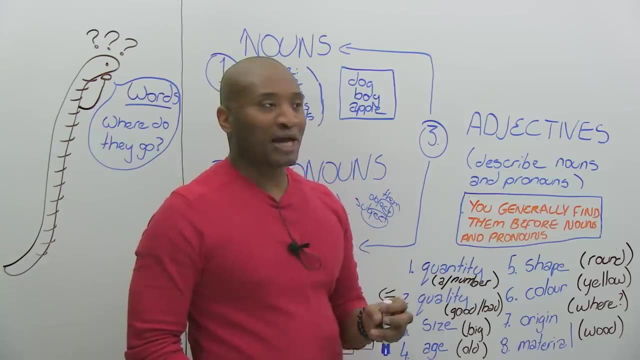 I don't even know. Yeah, I do. It's long and kind of circular, but, yeah, oblong. Colour: What is the colour? Yellow, black, green, red, Red? What's the colour Origin? Some of you go origin. 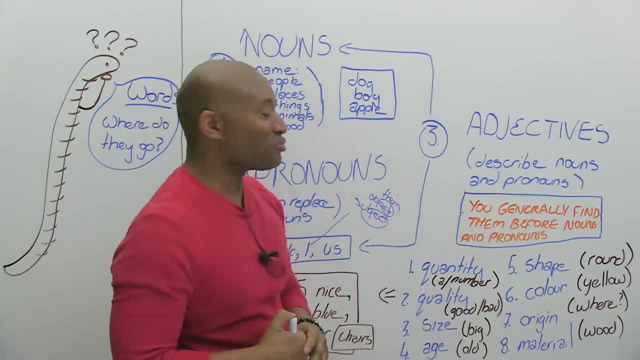 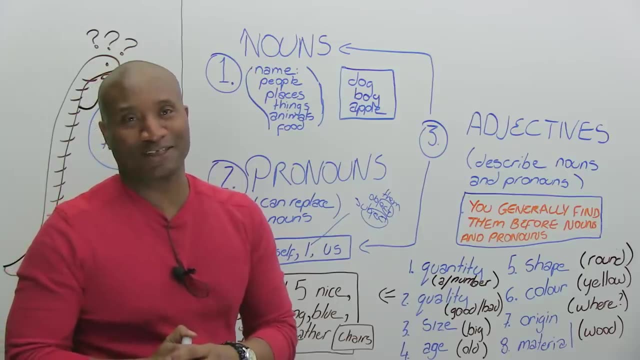 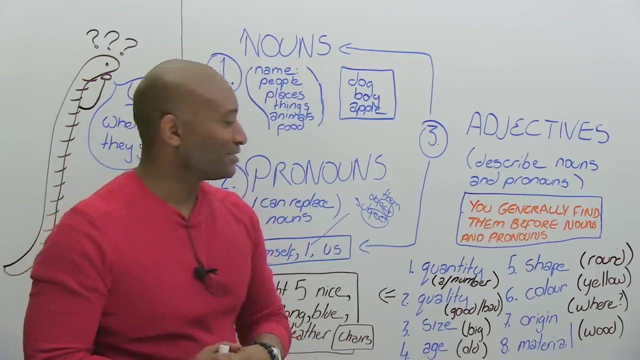 Wolverine origin Schnicked. No Origin means: where did it come from? Was it made in Italy? Was it made in China? China, Sorry, That was my favourite impersonation of somebody who goes China. I love China, China's good. 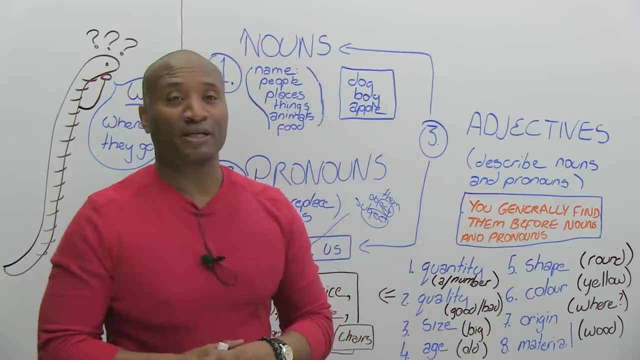 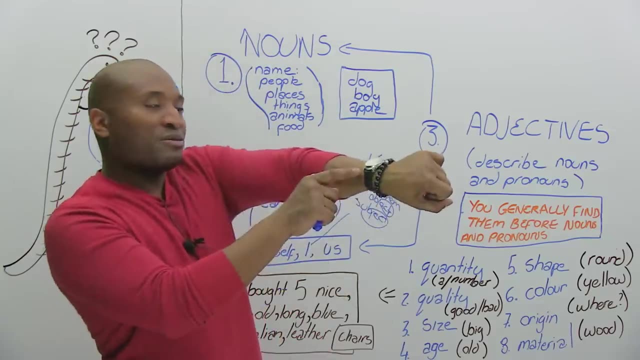 Anyway, Was it made in China? And what is the material? Is it cotton? This is made of cotton. Is it made of beads? So glass, Is it made of metal? I mean, you might not be able to see this, but metal. 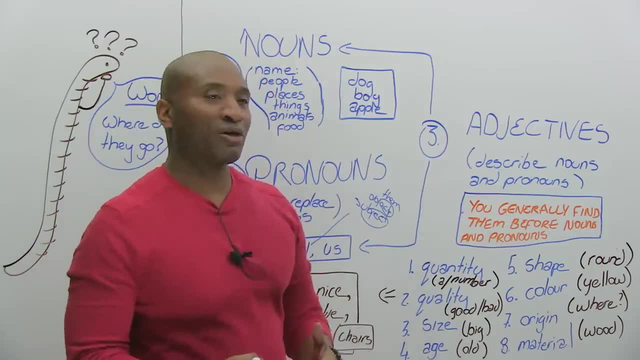 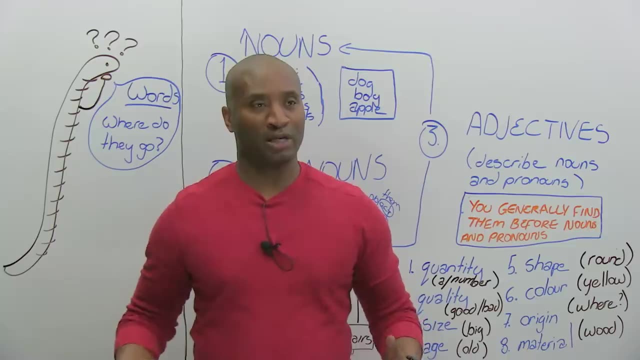 What is it made of? Okay, That is the order that we follow when we describe things, and I have an example that I've been hiding from you, that we're going to talk about, to show you exactly what I mean. So Mr E and I wanted to buy some couches, and Mr E was very specific on the kind of 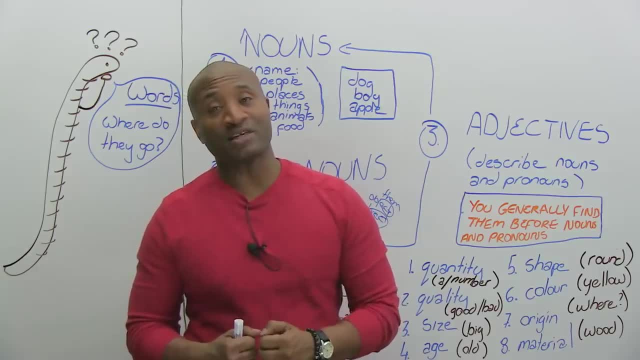 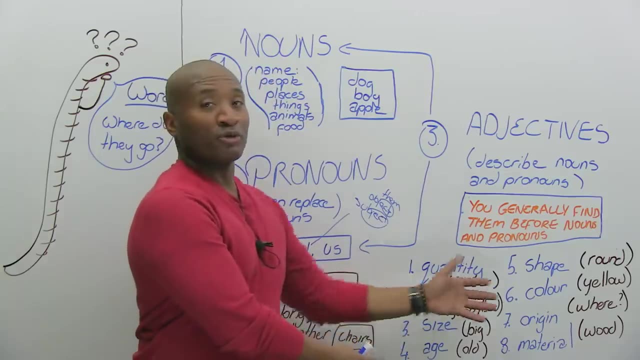 couch he wanted. so he gave me a list, And from that list I was able to get him exactly what he wanted. And how was I able to do that? Well, I followed the word order chart. So let's go take a look at what Mr E wanted. 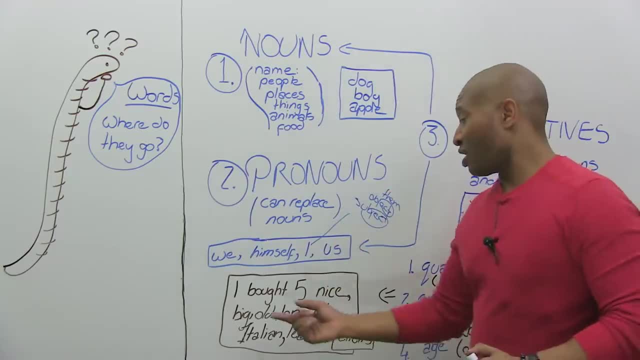 So Mr E wanted some couches and I said to him: hey, I got your couches. I bought five nice, Big, Old, Long Blue Italian Leather, Oh, chairs, Couch, Sorry. And Mr E said: fantastic, because if you had bought me nice old, big, long five, 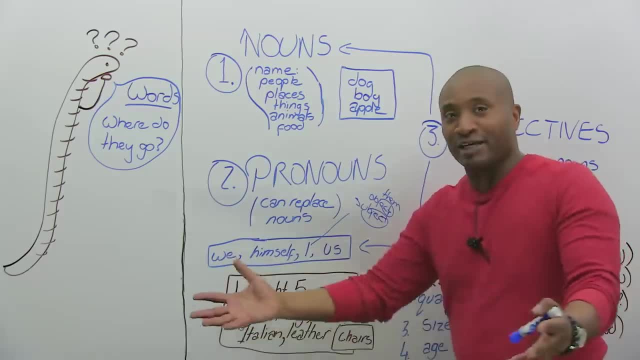 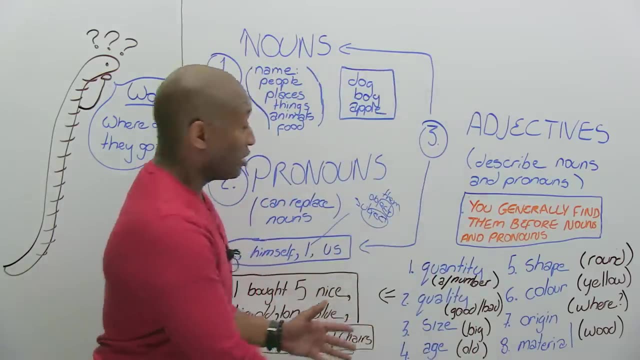 blue Italian couches, I would be confused and return it. And I said no, Mr E, because I know how we're supposed to order adjectives in English. So I followed your instructions by following the word order These five. 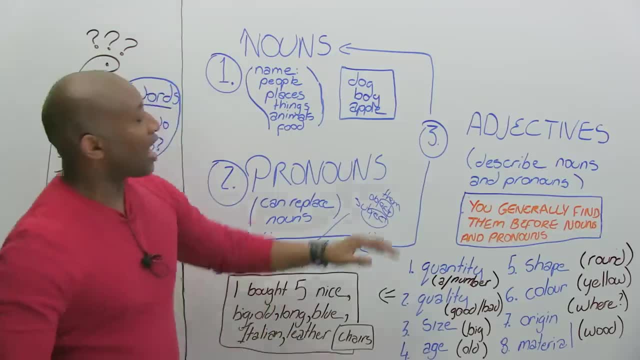 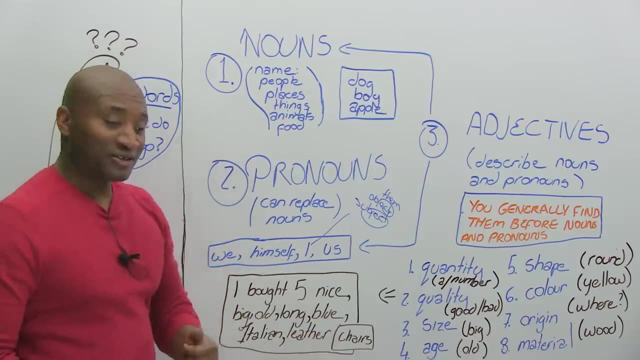 These sorry eight positions order, and I made sure I put the adjectives before the noun so I would get the exact right thing you wanted. Okay, So this is the first part of this lesson because I want to talk about. Now that you are a person, place or thing, you've got to do things right. 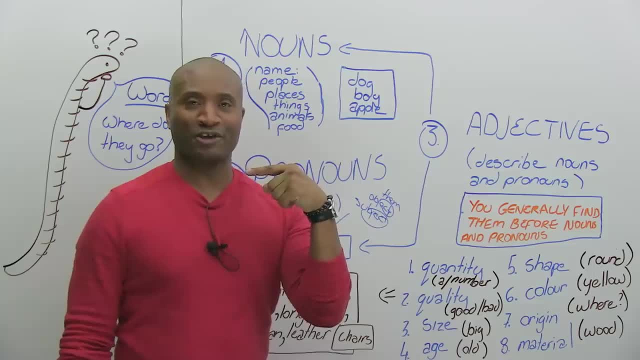 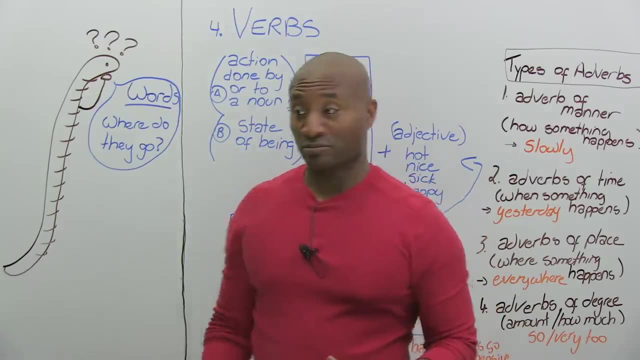 Like, right now I'm talking, which is a verb, which we're going to go to in a second, and talk about verbs and how they work. Are you ready? Okay, Well, we talked about nouns, pronouns, adjectives, how they work together. 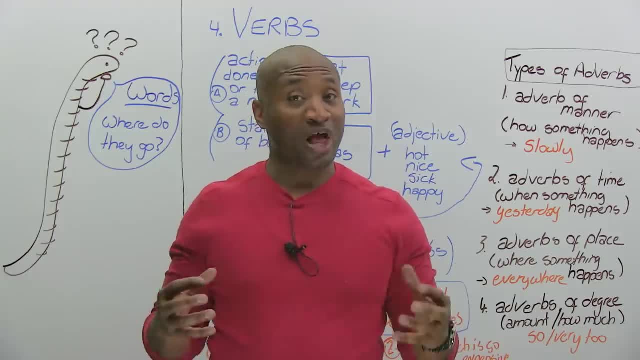 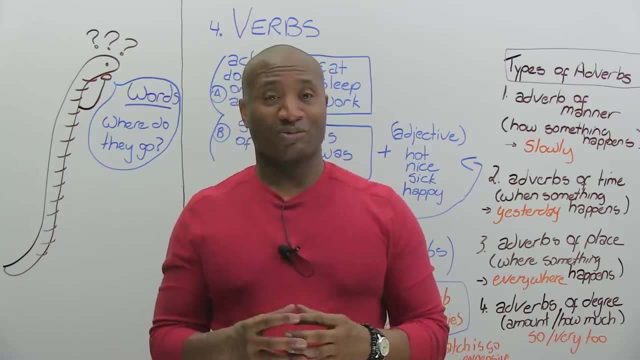 Remember, a pronoun can replace a noun. The order that they come, right, They come in. And now I want to talk about actions, because a noun or a thing that doesn't do anything is rather boring, right, Wouldn't you say? 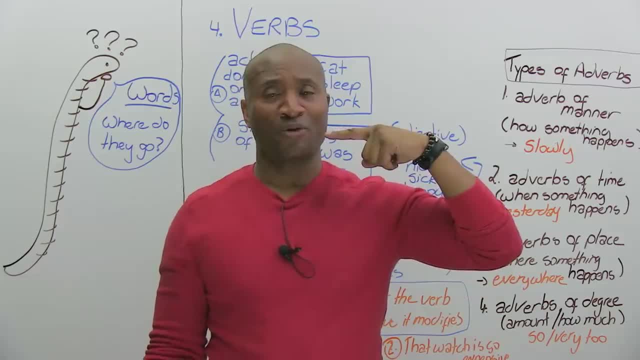 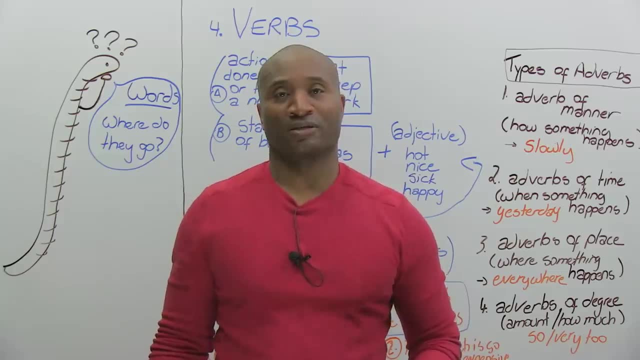 And what do we mean by actions? Well, right now I'm talking, My mouth is moving, I'm talking, But I'm also looking at you. I'm breathing, okay, So let's go to the board and look at this funny word we call verbs and how they work. 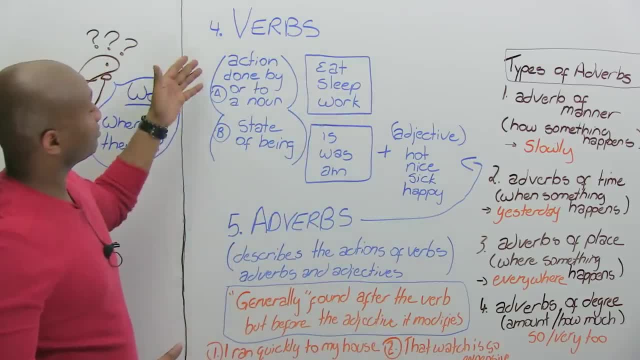 Well, with verbs we have. Well they do actions right, We take a pronoun or a noun and they act. They can sleep. Did I just press eat and sleep? They can eat, sleep and work Okay. 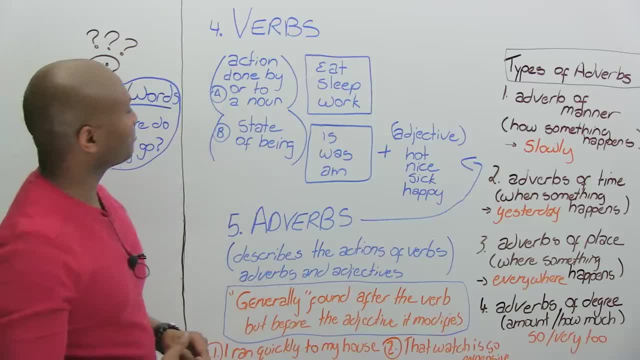 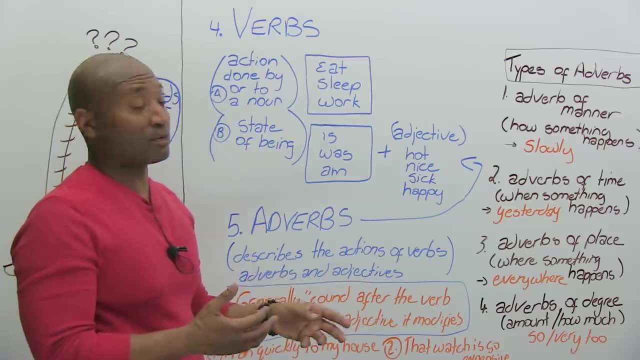 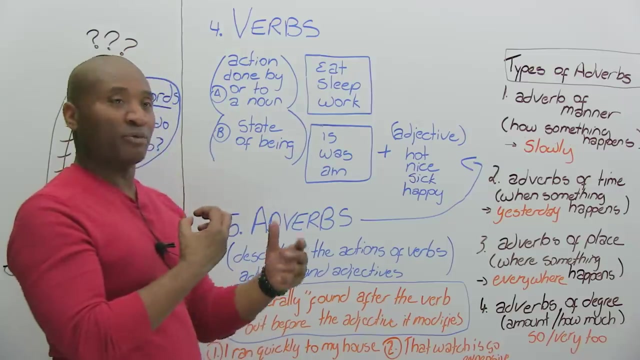 So that's what a noun can do And we talked about, you know, subjects and objects pronouns The subject pronoun does it to an object pronoun. okay, One of these actions. So I eat an apple. I am the subject: eating an apple object. 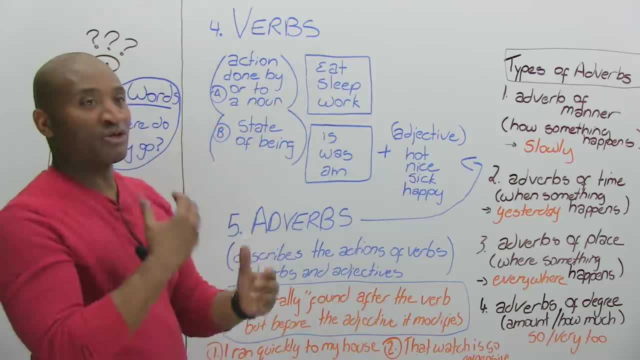 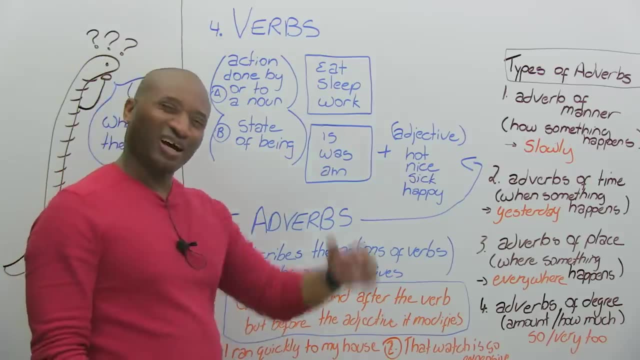 Cool, So we put this word here, the verb, to tell you how the two things are working together. Here's a funny one. Verbs are state of being, Huh, Huh, Huh. Being what Well exists. 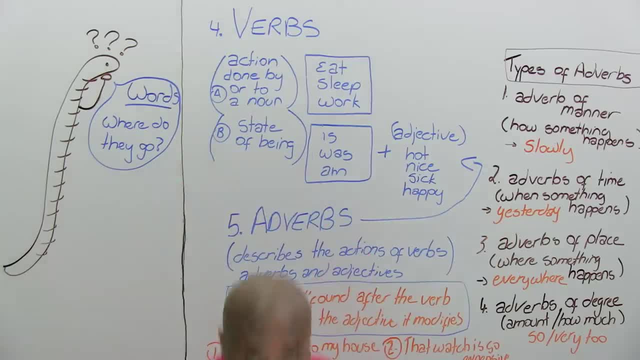 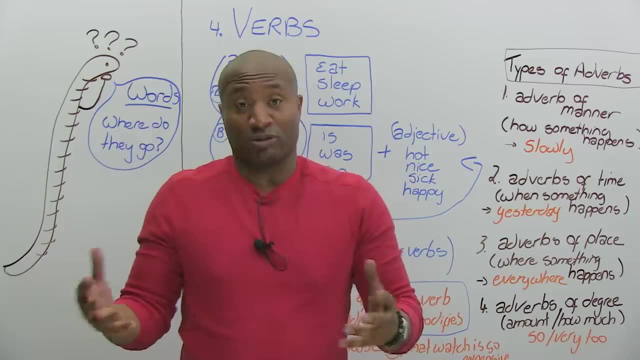 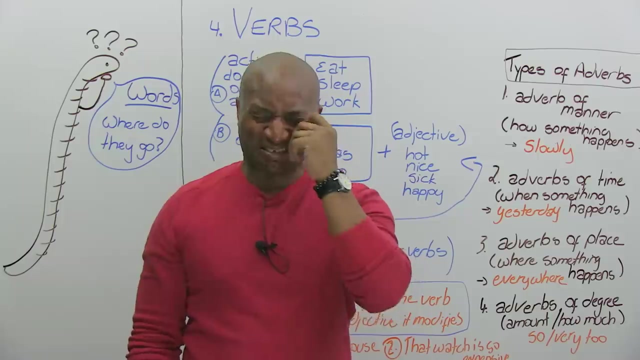 Like right now I exist. If I stop being, I disappear. So being means you are there, you exist, you're real, you can be touched. But it's not just that. Sometimes I'm happy, Sometimes I'm sad. 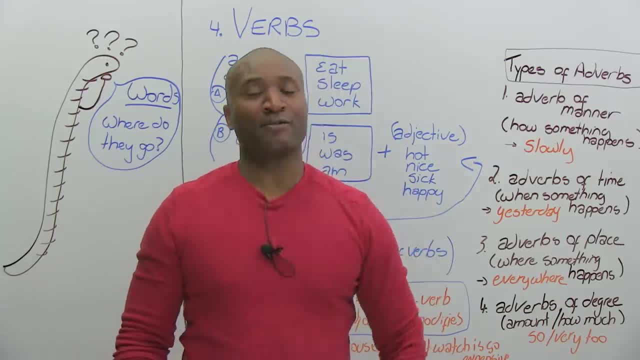 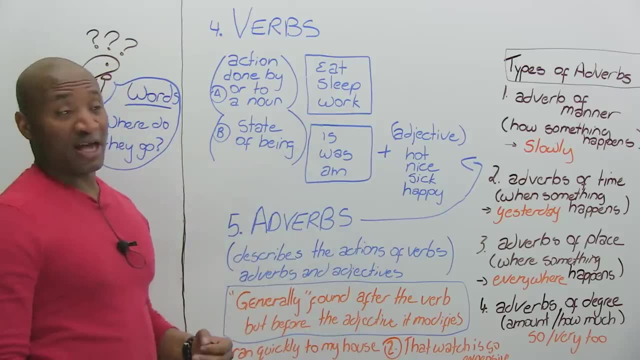 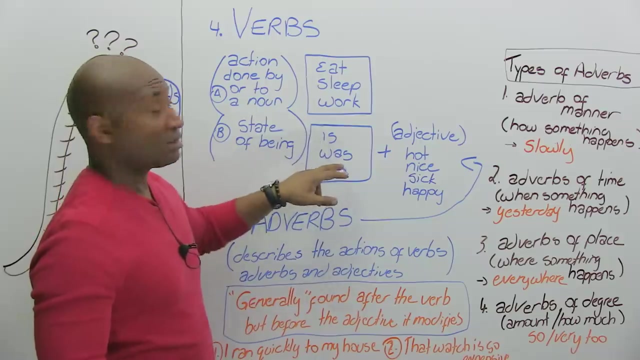 And sometimes I'm sick And sometimes I'm healthy. You'll notice that we use the verb to be to talk about those things I am, she is, they are Okay, And we can use that, this verb to be with an adjective, and it tells us how something. 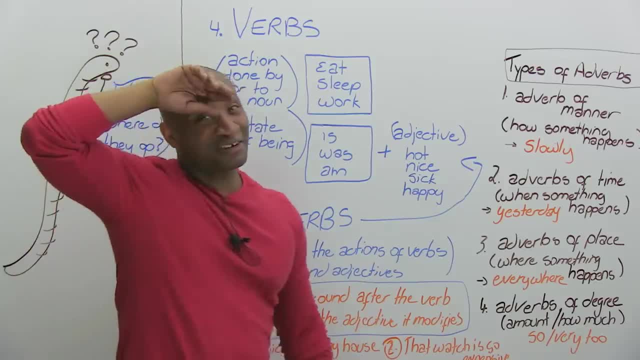 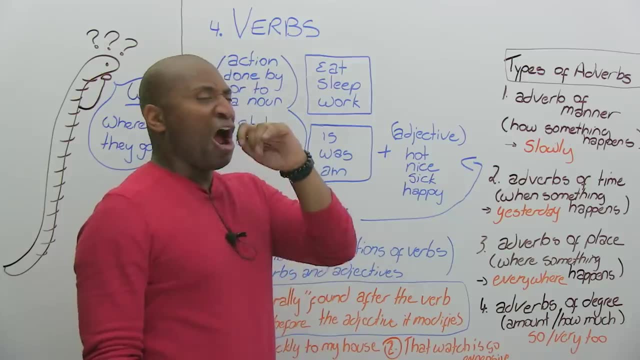 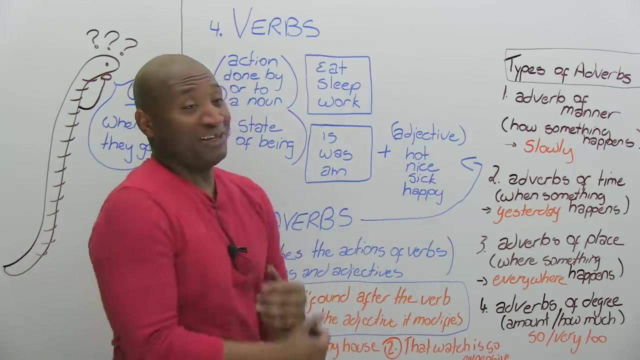 is right now, Like right now, it is hot in here. Hot, That's the state of the situation or how things are right now. Right now I'm a little sick. James is sick. That's my state of being And I'm very happy when Mr E comes to my house. 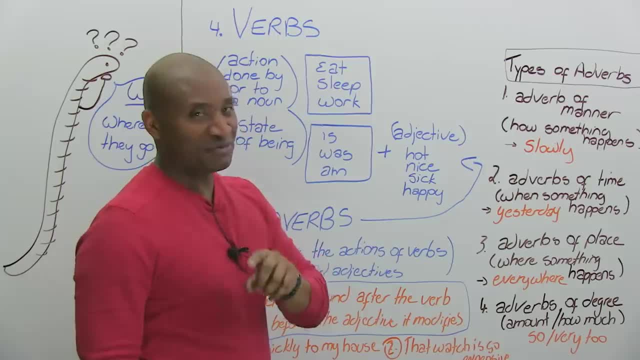 Right, You didn't see him, but I mentioned him in every video, So I'm happy. That's the state, or how I am, or how I'm feeling my emotions. You are happy, sad, upset, exuberant, which means very happy. 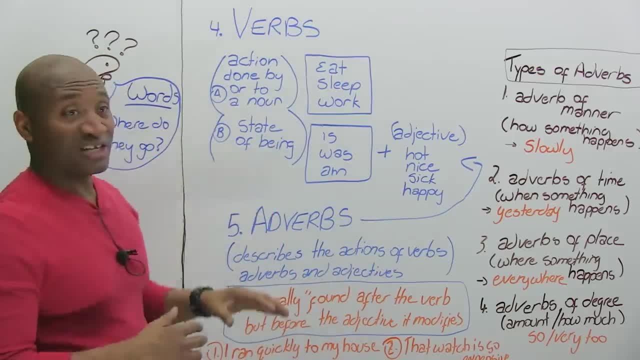 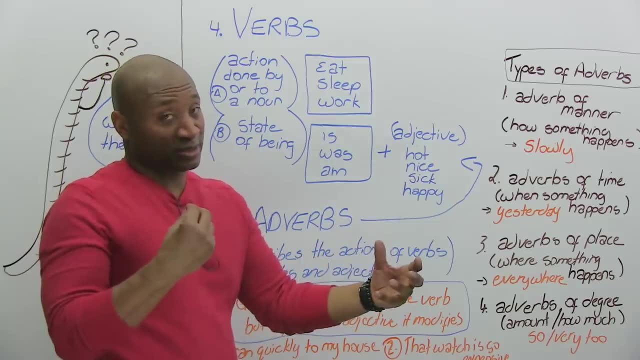 Okay, So this is what verbs do. They can tell us the action One noun is doing to another noun. In that case, we talk about subject and object pronouns, Right, But we can also talk about how things are. The world is good. 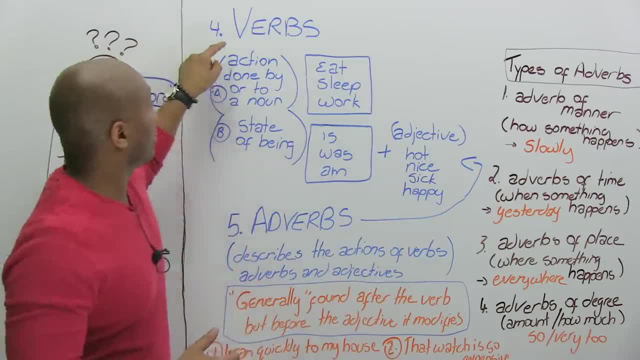 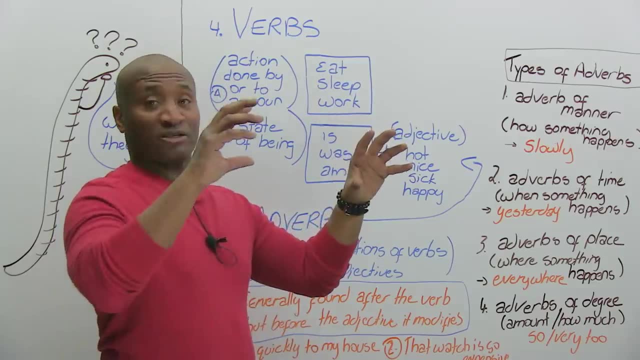 How it is Cool. Let's move down from verbs to adverbs. Do you remember when we talked about adjectives and we said add toject, and that was because you have subject and object? Well, we have the same thing here. 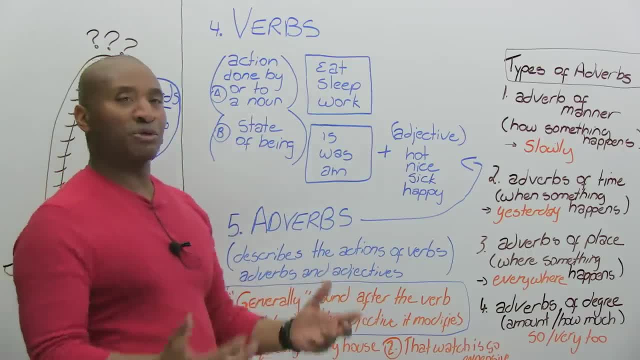 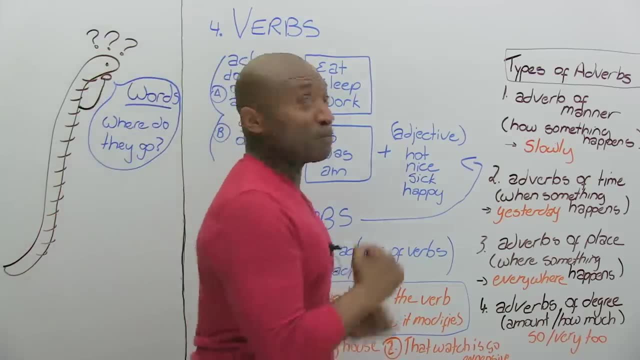 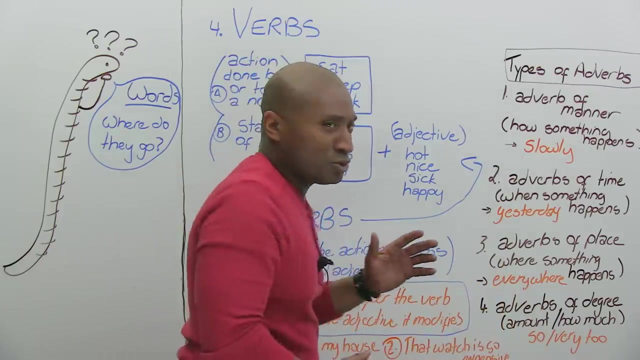 We add to verbs, Which means we give more of a description. We give more of a description of what the verb is doing. It's one thing to run than to run quickly. That's different, It's not the same. Or on do-do-do-do, do-do-do, Bionic Man style, slowly, but really quickly. 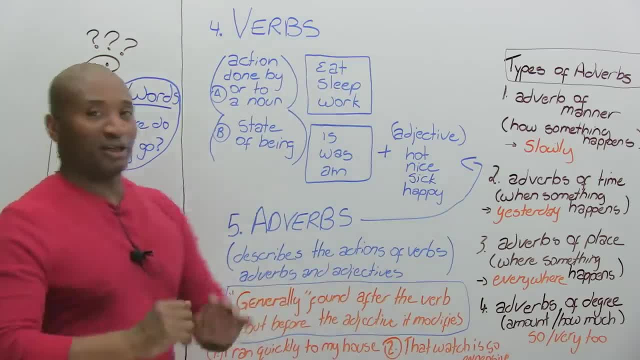 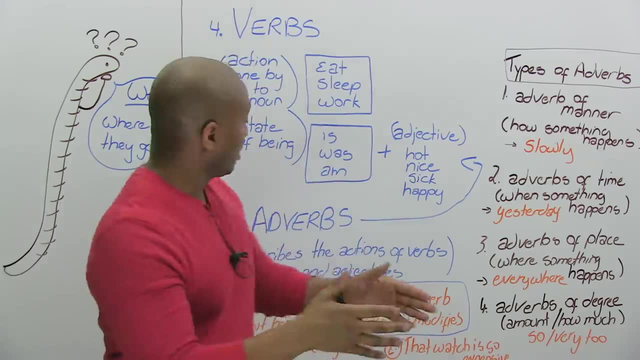 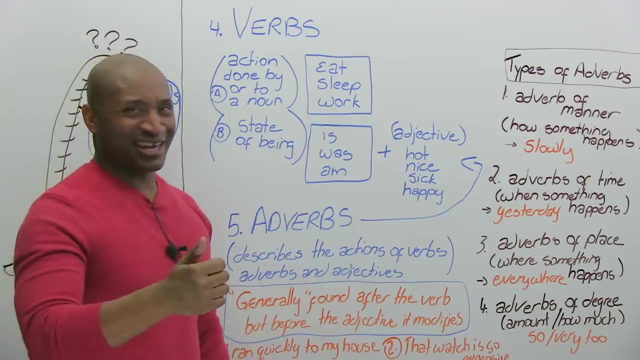 Okay. So adverbs describe the action of verbs. but hold wait. Unlike an adjective that just describes the pronouns, Adverbs describe verbs: okay, adverbs okay and adjectives: This adverb is very, very busy. 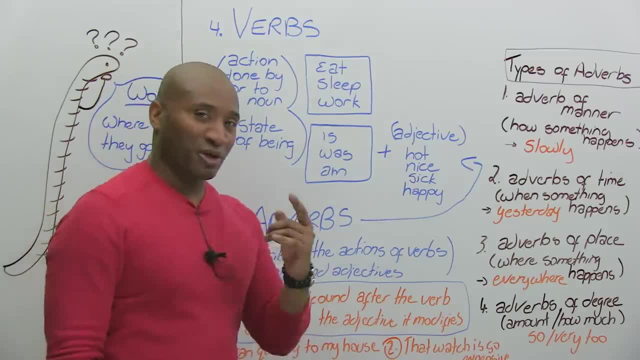 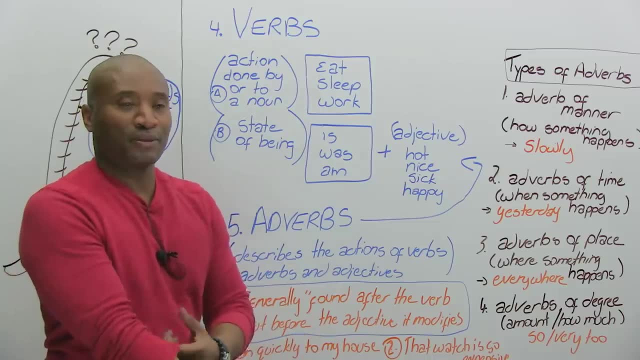 It's got a lot of work to do and it's going to be my job to show you how it does that work. An adverb is interesting because it adds information to how things are done. In doing that, first of all, we should talk about its position. 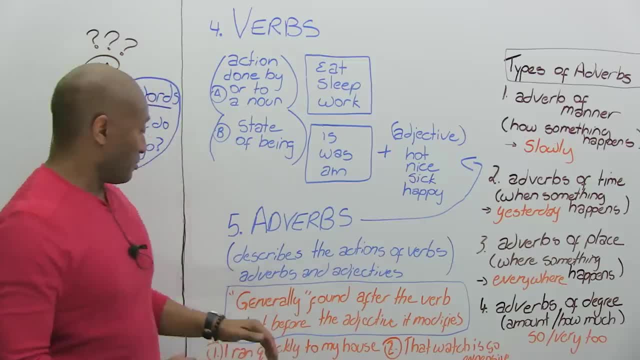 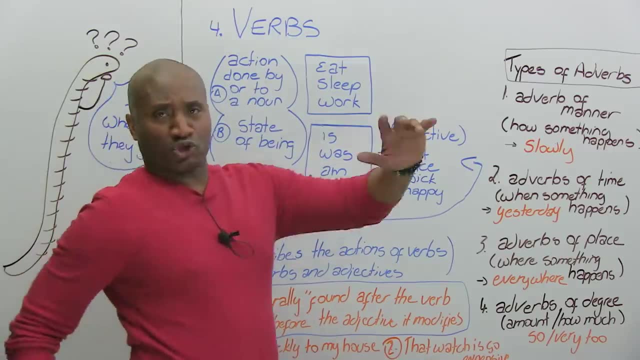 Generally, Adverbs are found after the verb but before the adjective. it modifies. so let's do one at a time. Do you remember? I was running and I said I'm running slowly or I'm running quickly-quickly-quickly-quickly. 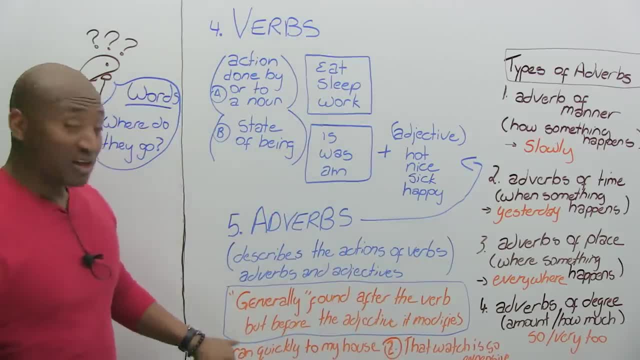 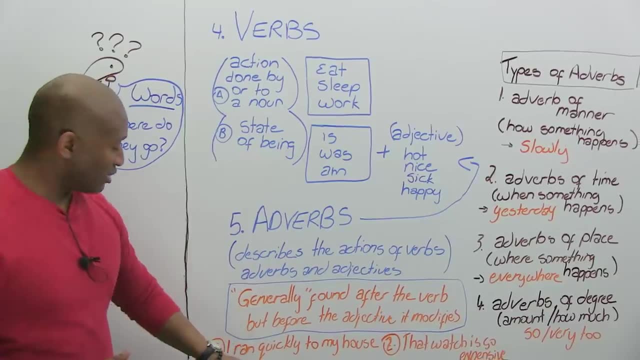 In this case I ran. I want to know what the noun or pronoun is doing and then how it ran, So in this case, ran quickly. Okay, Notice, it follows after the verbs. This is generally true, Okay. 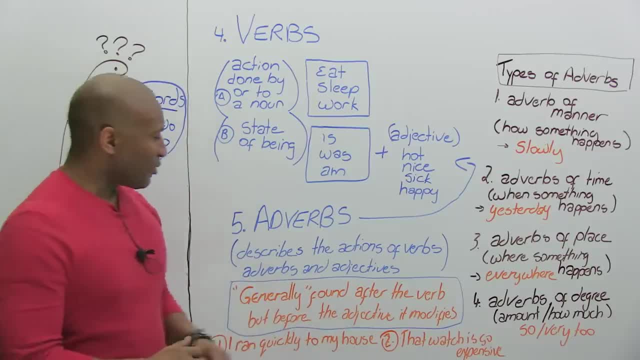 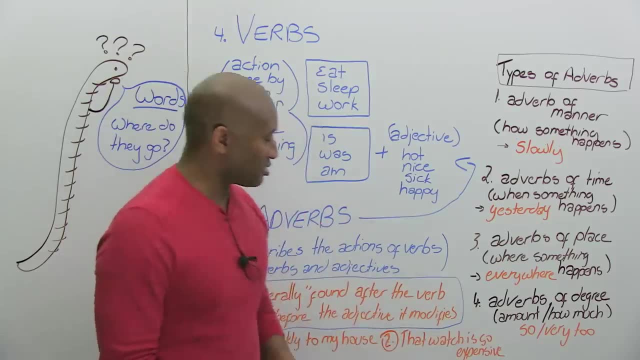 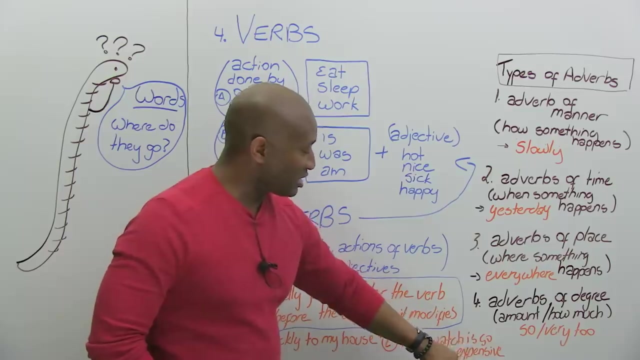 So I ran quickly to my house. Now I talked about adjectives and I don't want it to get too complicated, but I'll show you here That watch is so expensive. Hmm, Well, that watch is the subject we're talking about and we're saying is expensive. 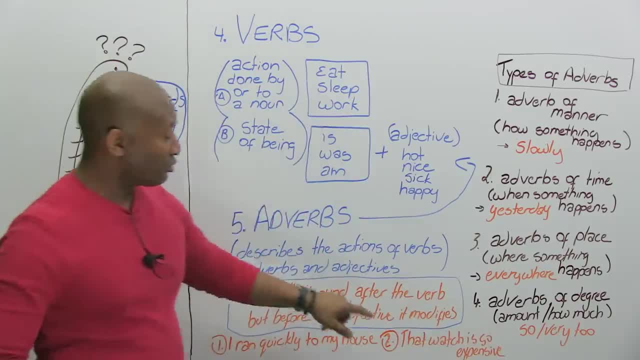 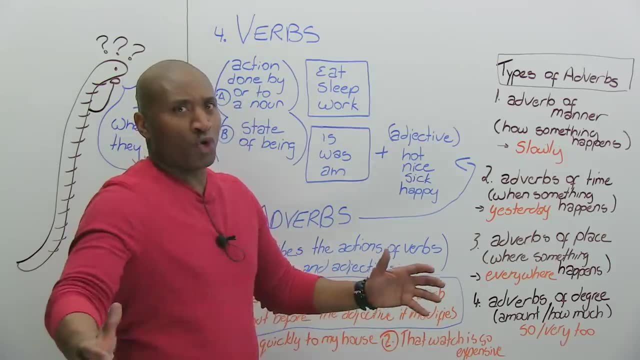 If I get rid of so. remember we talked about stative verbs. We're saying: the watch is expensive, Right, But how expensive is it? I don't know. It's so expensive, Okay, It's so expensive, which means very expensive. 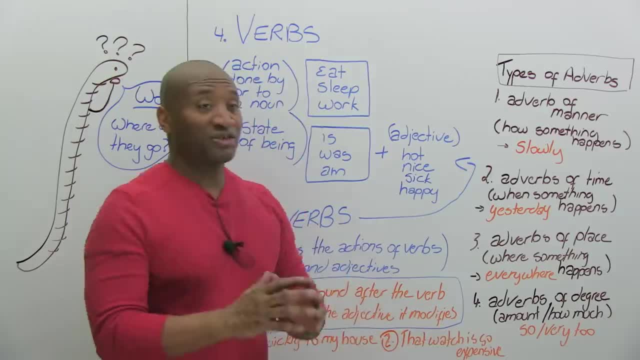 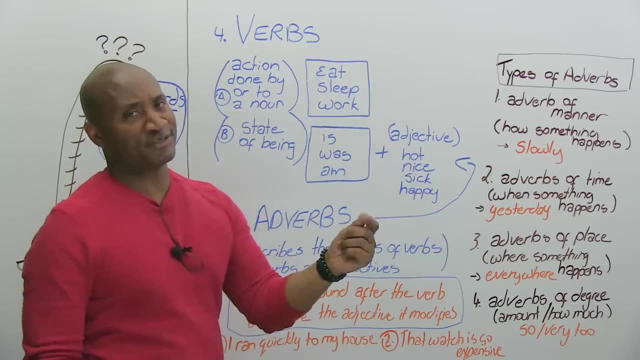 So we actually use an adverb to describe, to tell us the degree or the amount of expensiveness. It's very expensive. That means a lot of expense. You need a lot of money to get that watch. So adverbs help by noticing. it's still following the rule following the verb, but it helps. 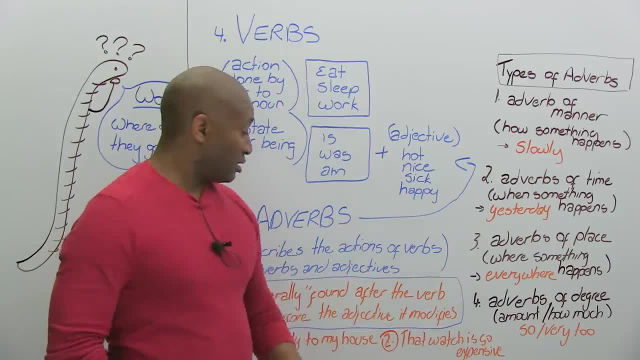 to give more information about the adjective which is telling us about the watch. So adverbs are really cool because they make everything better- Cool Me too. But what I want to let you know is there's something else about adverbs. 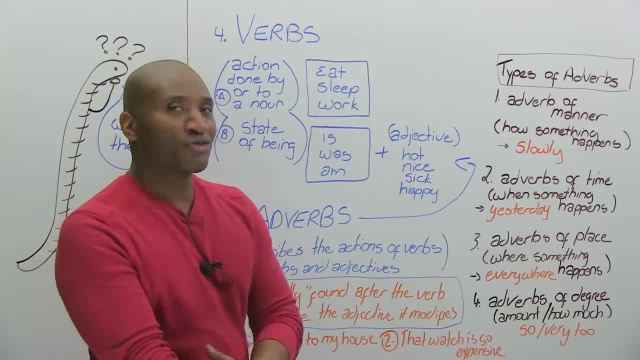 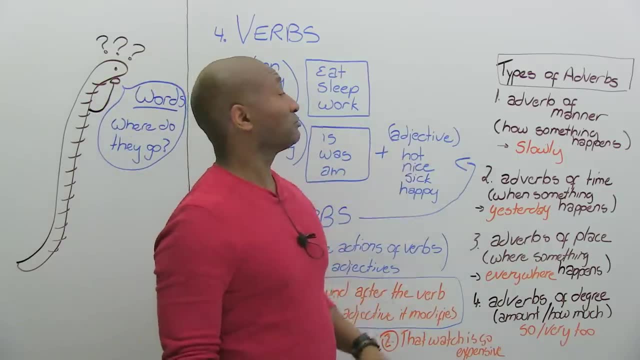 There's not just one type of adverb- Uh-uh, uh-uh, There are four, And let's take a quick look at what the four are: The types of adverbs. we can talk about number one. we can talk about adverb of manner. 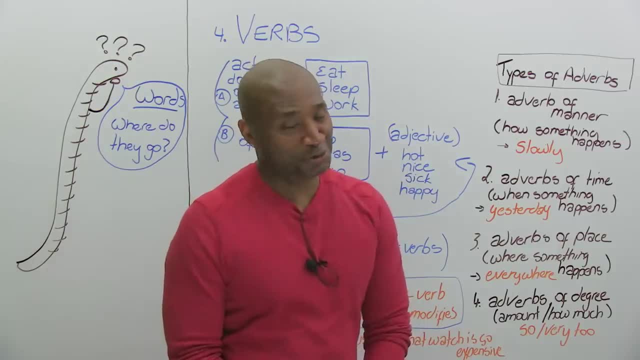 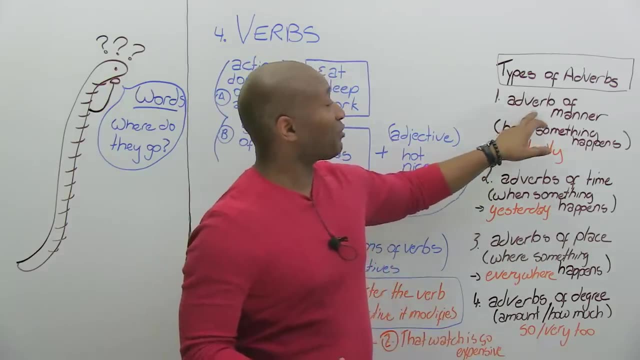 Please thank you. that's so kind of you and you're welcome. No, I'm not talking about adverbs being polite and nice. What I'm saying is, When we say adverb of manner, it is how something happens. Some things happen slowly. 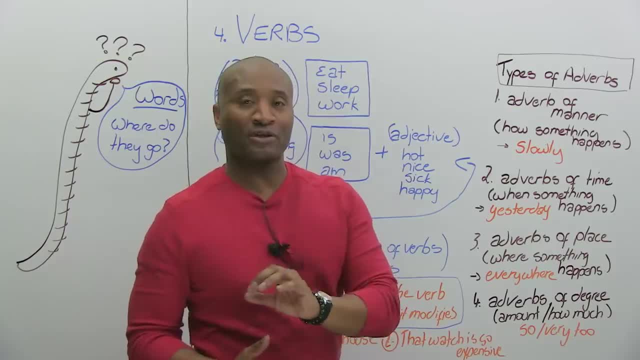 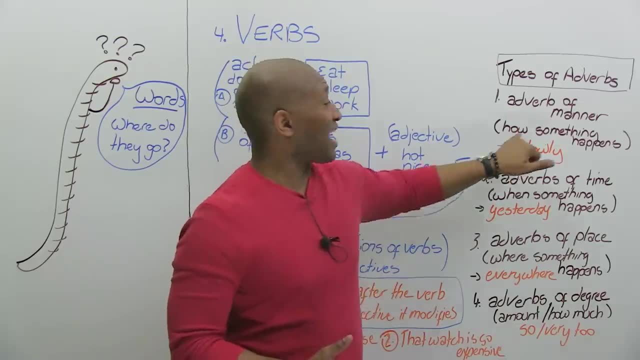 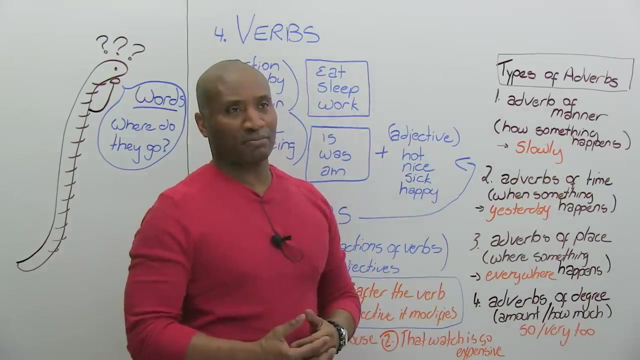 Some things happen very quick. They happen very quick or fast, Right. So in this case, when we say: how did it happen slowly, quickly, that's how it happens over time, Right, Adverbs of time: This is when something happened.